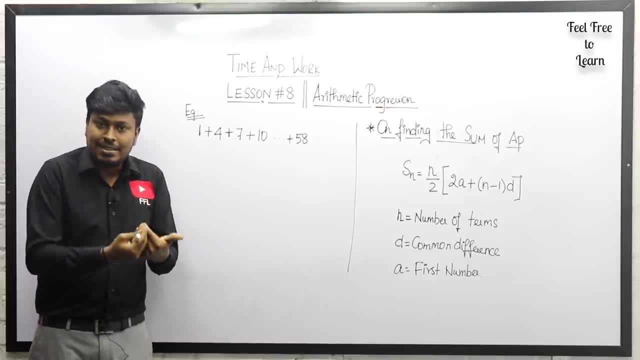 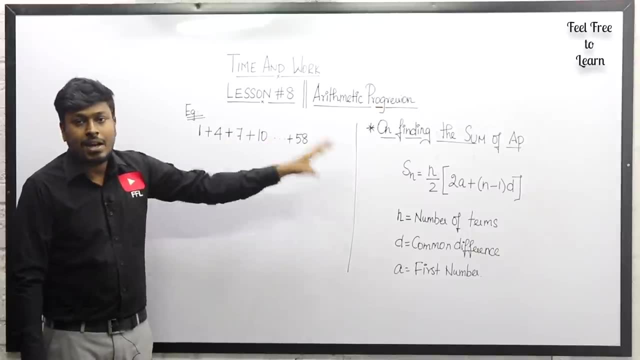 So here the questions. right after reading certain number of questions you can see there will be some sequence form like this. So we need to solve the sequence only by an arithmetic progression logic, no other way. So, friends, listen here. First let me learn. 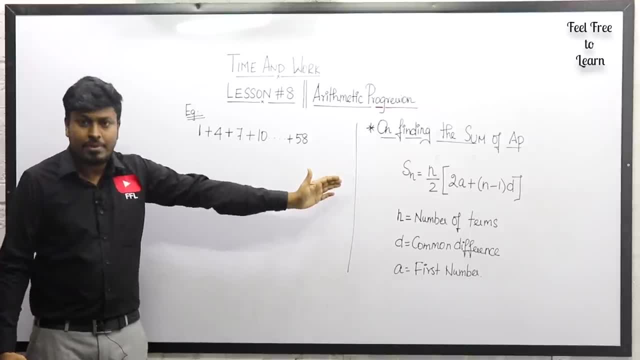 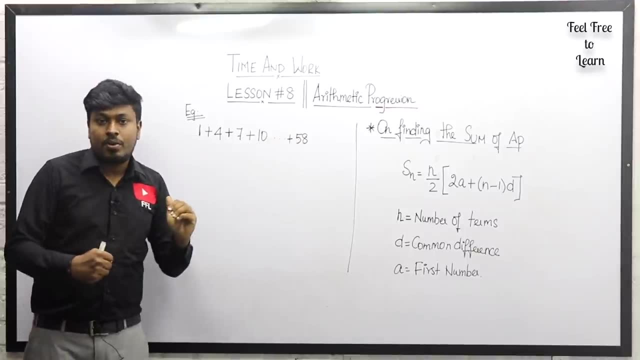 what is called as arithmetic progression Formula, And then we can learn how to apply this in the basic example right. So, on finding the sum of arithmetic progression. usually arithmetic progression is a series, like it looks like a number series. right, By seeing that series, we need to find the sum for the 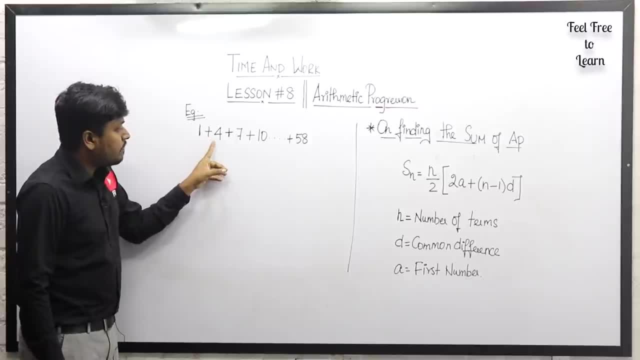 total. For example, let's let me take, see here, 1 plus 4, plus 7 plus 10.. And it goes on till 58.. It's in the sum logic, right? So 1 plus 4, they have added 3,, 4 plus 3,. 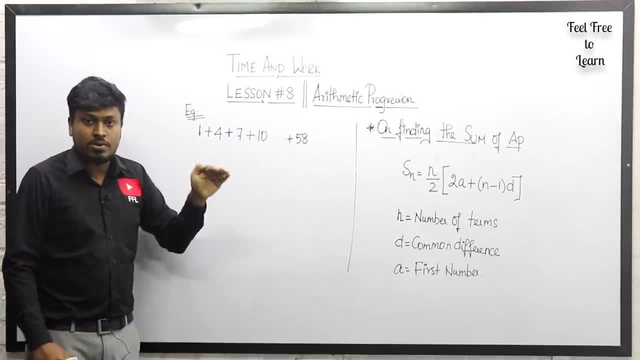 7,, 7 plus 3,, 10,, 10 plus 3 will be 13,, 16,, it goes on till 58.. So our target: to find what is the total sum. If we need to sum, we need to find the sum. what we need to do in the basic, traditional method we need: 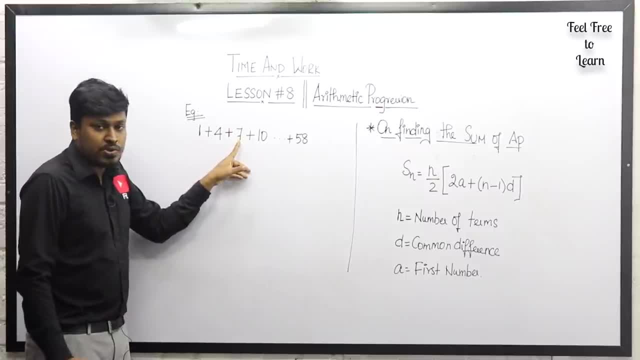 to add: 4 plus 1 is 5.. So 5 plus 7 is 12,, 12 plus 10 is 22.. So we need to add all the numbers. So it is not an easy way, right? If it is 58, we need to add till 58. So in order to do, 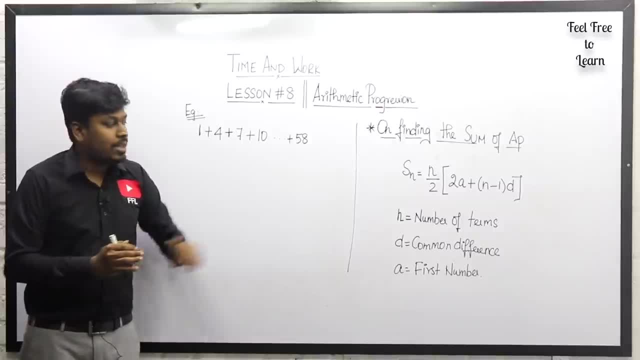 that we have a formula in arithmetic progression. If we use the formula, we can able to find what is the sum of this. AP understood So arithmetic progression. you know in the childhood, in 10th standard or 9th standard, we would have already learned what is called. 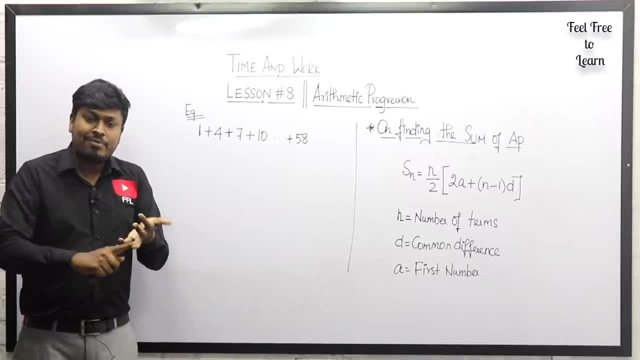 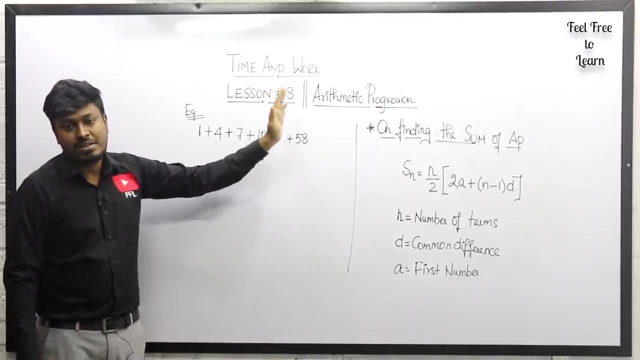 as arithmetic progression, geometric progression. we have many formulas in arithmetic progression, But here I'm going to teach you only one formula which will help to solve a question in time and work. that is enough. right? We are having many formulas in arithmetic progression. we 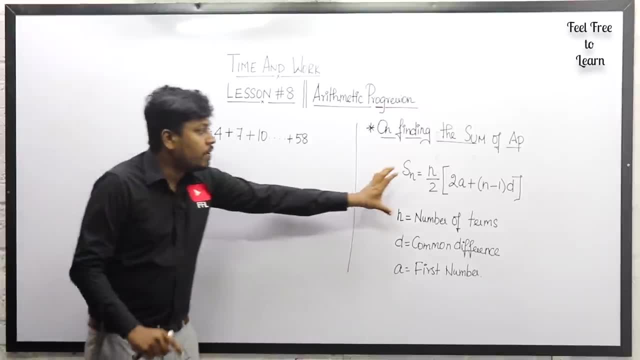 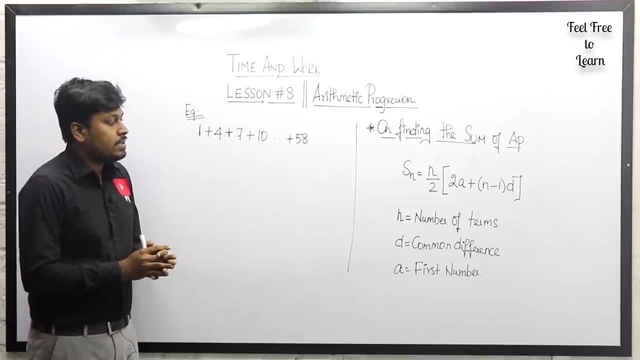 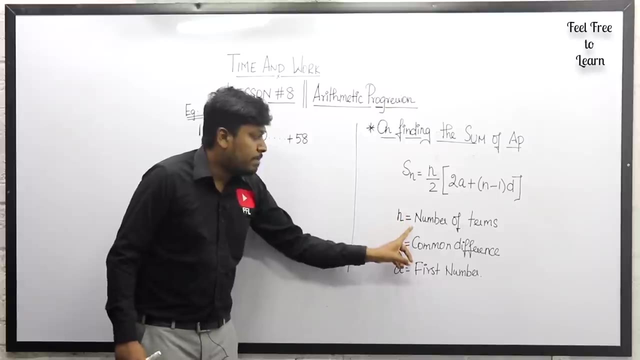 don't want to learn all those formulas, Only one formula. this formula is enough to solve a question in time and work based on the certain logic understood. So the formula is: S of n is equal to n by 2, 2a plus n minus 1 into d. So here, where n represents the number, 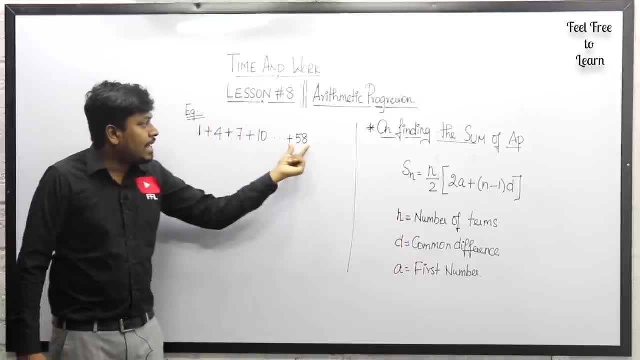 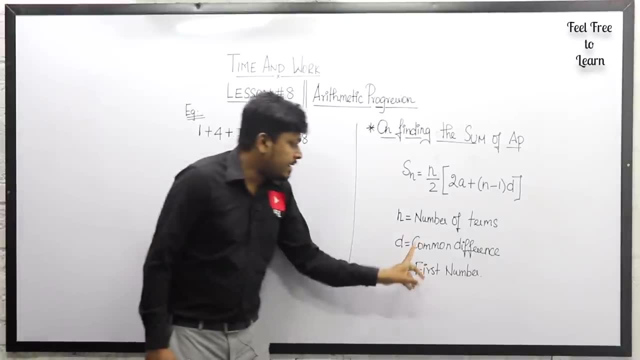 of terms here. how many terms are there, Starting from 1, it has 58 terms, So the number of terms will be given. So instead of n we will use the total number of terms. And second is d. d is the common difference. Difference between 1 and 4 is 3.. Common difference for: 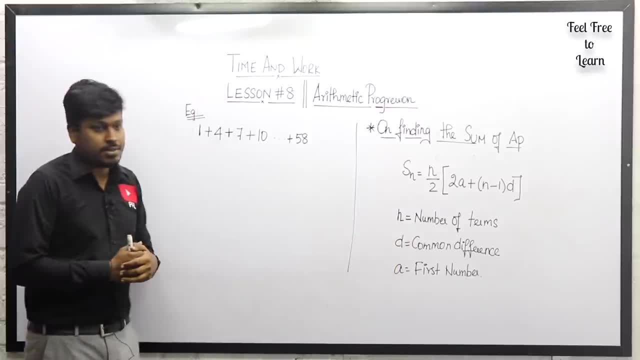 1 is 3, understood. So d represents the common difference And a represents the first number. So here the first number is 1.. So instead of a we substitute the value 1, understood. So that's it. we will apply all the values in the formula by using the series First. 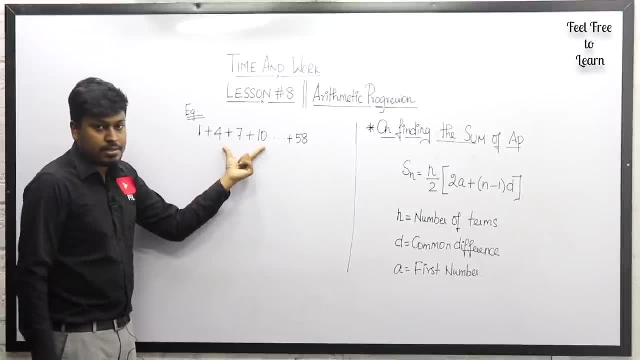 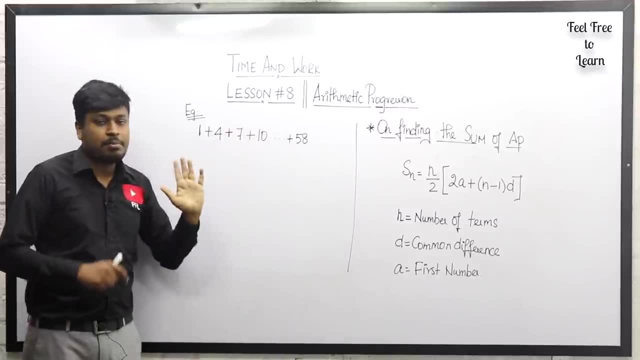 after reading time and work question we usually form the series. So after forming the series by taking all the numbers, difference, last number we will substitute in the formula and we will find the sum of the total a, b understood. So another important thing is that we are going to solve a question in time and work based. 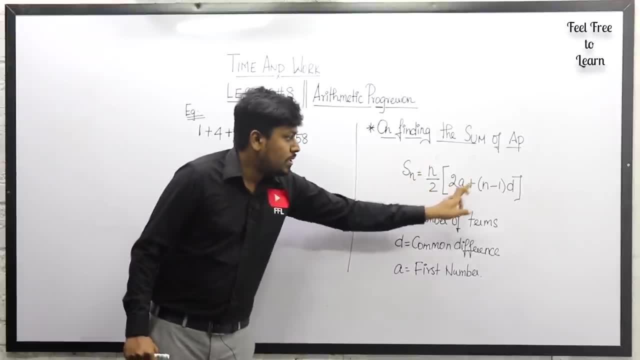 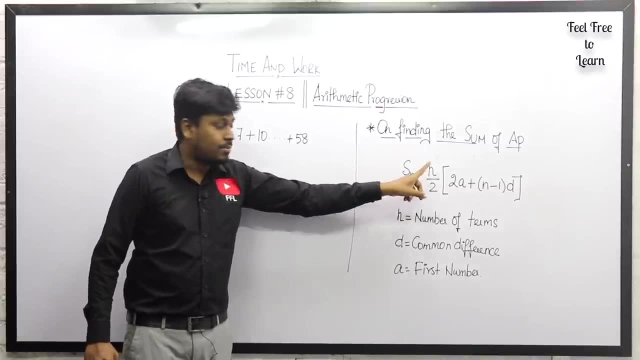 on that. d Second important thing is here you can able to see 1,, 2,, 3, 4 values are unknown understood. 1 is s of m. sum is unknown. Second, n is unknown value And a is unknown value. d is: 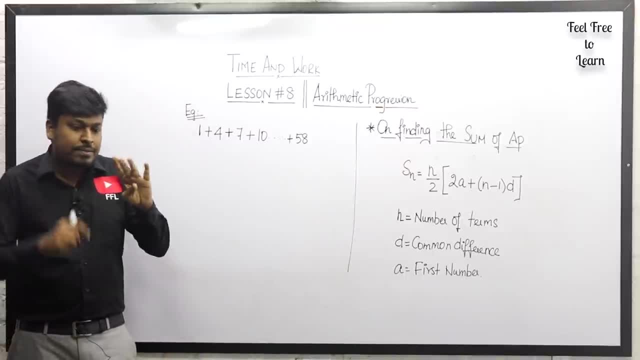 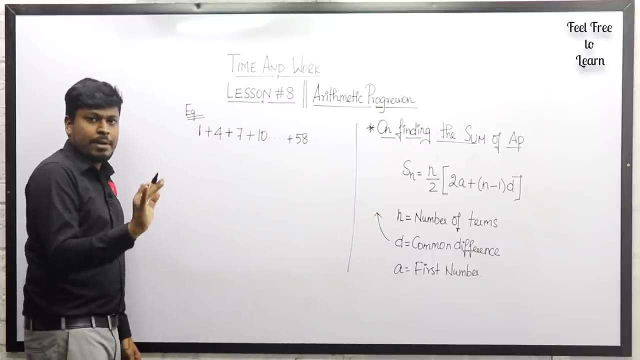 unknown value. So after framing a series out of 4, definitely we will know 3 unknown values. So our target: to find one unknown value and we will find the answer right. And second important thing is just see the value of d is called as a difference, right. 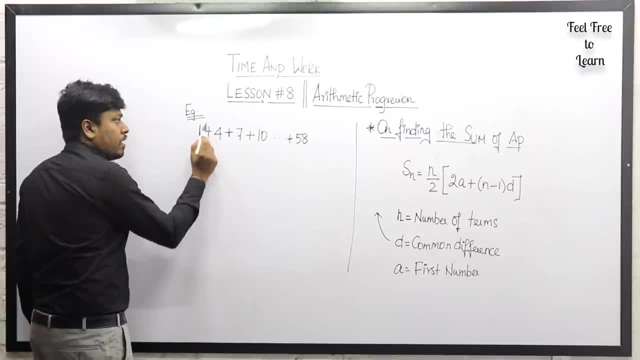 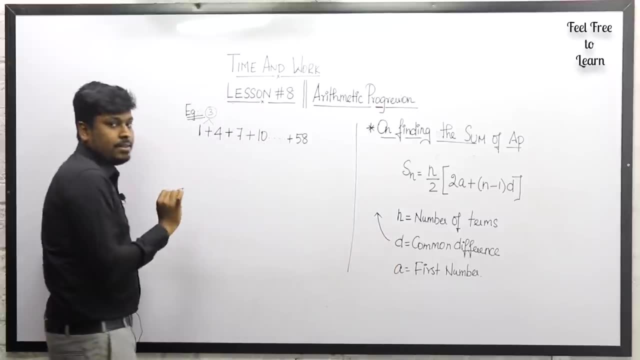 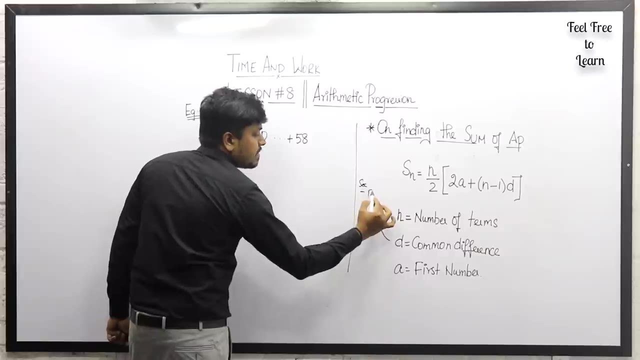 difference. for example, here we have one, here we have four. so the common difference between one and four is three. yes, so here, instead of D, we will put the number three. but logically, remember one thing: so the value of D is second number minus first number. understood? what is the second number here? four? what is the? 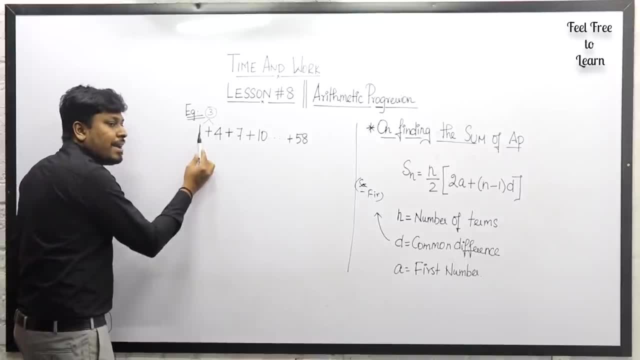 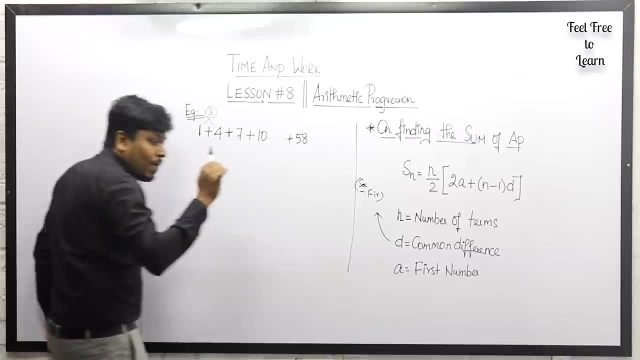 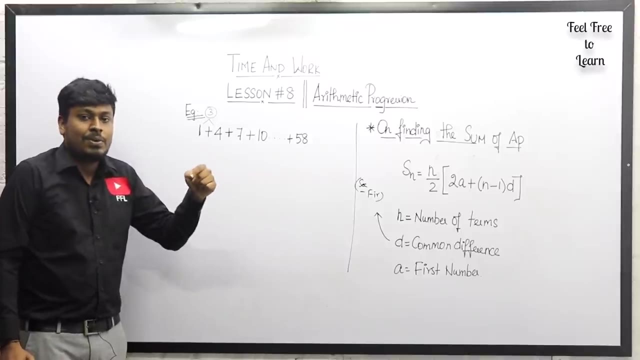 first number here one. so second number minus first number. four minus one will be three, understood, keep that in mind. D is called as a difference, but anyway, remember this. D is also called a second number minus first number because if the numbers are in a descending order, in that scenario where most of the students 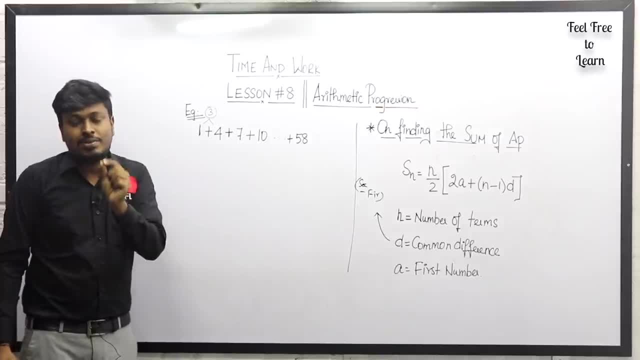 will make a mistake. that's what I am saying. the value of D is equals to second number minus first number, understood? so now what we can do is we can solve this series by the given formula, that is, arithmetic progression formula. see here, the starting number is 1 and the second number 4, 7, 10 and it. 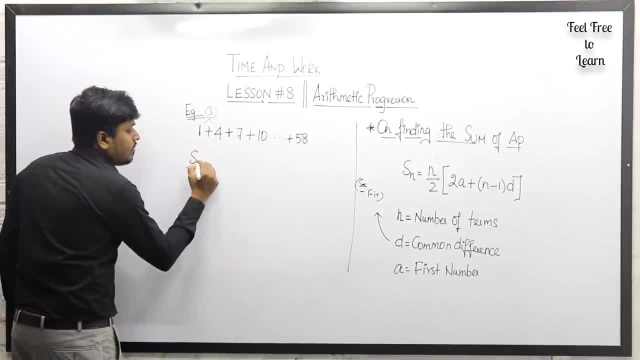 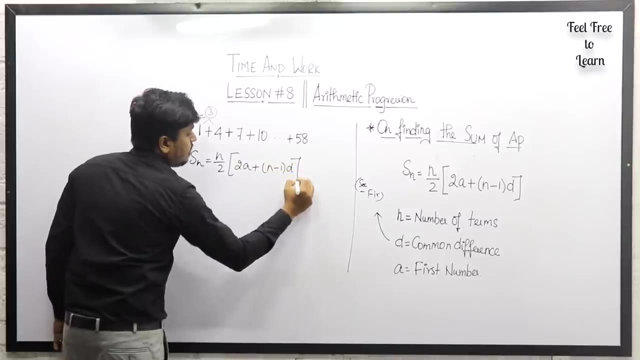 goes on till 58. so here our target: to find what is the sum of arithmetic progress, that is the total value sum. what is the formula, actual formula here? so S of n will be the total sum, right. so n divided by 2 into 2, a plus n minus 1 into D. so this is the formula for AP. and now we 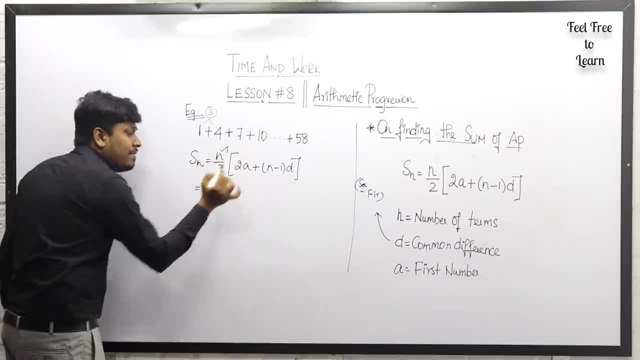 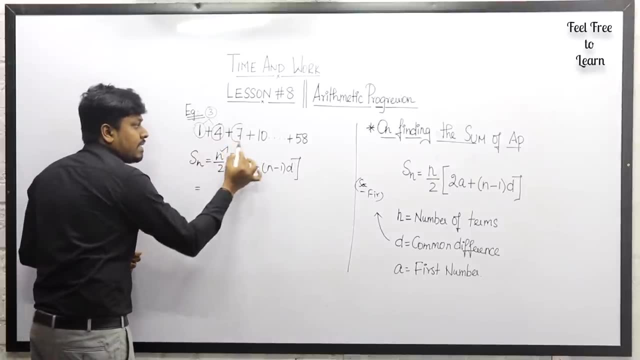 need to substitute all the values right, just see here. the value of n will be the number of terms, right number of terms which determines here: 1 is one term, 4, second term, 7, third term, 10, fourth term. till 28, we have 28. 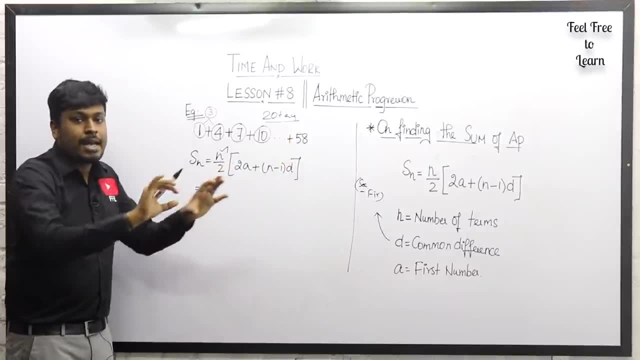 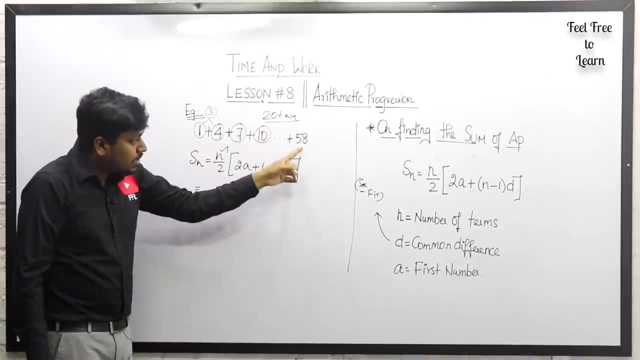 terms. so here finding is difficult, but while reading time and work question we can easily find how many terms are there. it's just an example. question, right? so totally, 1, 2, 3, 4 till 58. we have 20 terms. so instead of n substitute 20 divided by. 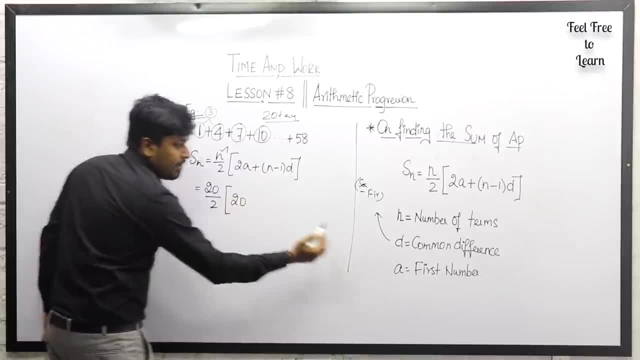 2. so into 20. so the value of a. so the value of a will be the first number, so a, the first number is 1. so 20 into 1. so 20 minus 1 will be 19 and the D will be the. 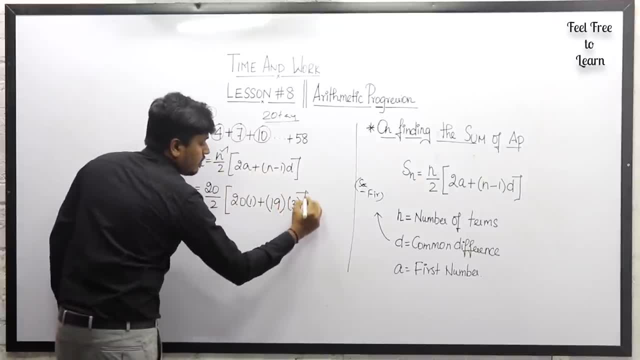 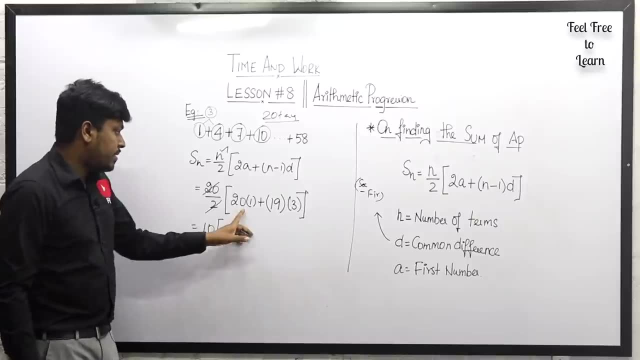 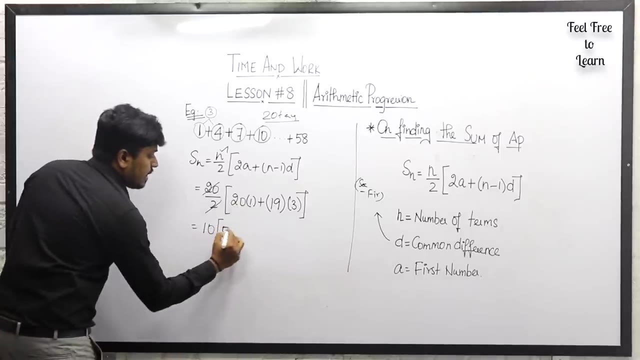 difference, so difference is 3, right. so now we need to substitute and cancel all the values. so here we can cancel. it becomes 10 here, so this will be 20, so this will be a 19, 3 and 20, which becomes 59, so 59 into 10, so the total sum will be 590. so this will be the. 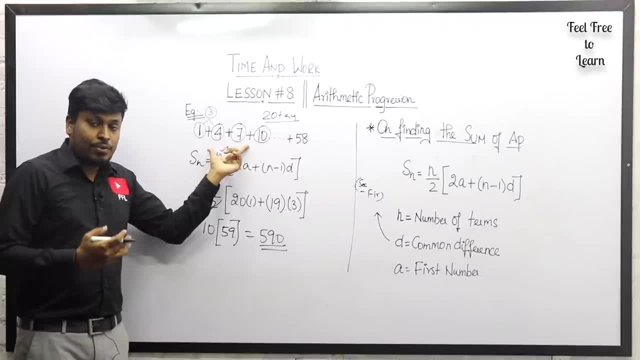 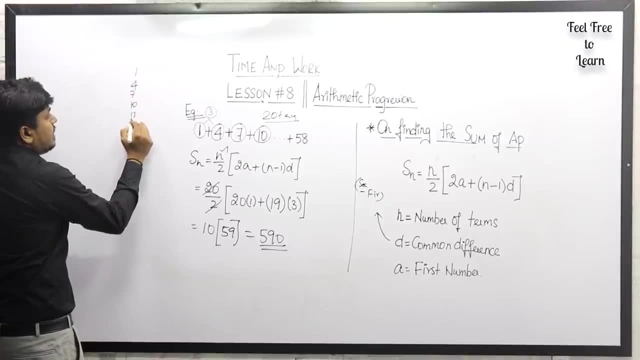 answer for this given example series: right, if you need to solve in a traditional way, right, it's a lengthy process. just see, we need to add like this: 1, 4, 7, 10, 13, 16, 19, 22, so we need to write all these numbers until 58 and we need to add all. 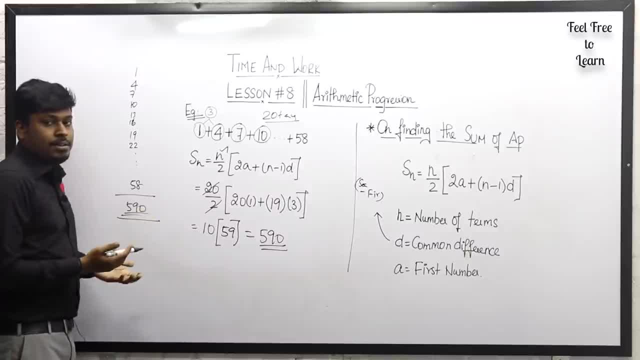 the values. here also, you will go in to get only 590, right, so it's a traditional method. but this, this won't help you even in childhood, right? so because it's a lengthy process. that's the reason they have given an AP formula, so use this AP. 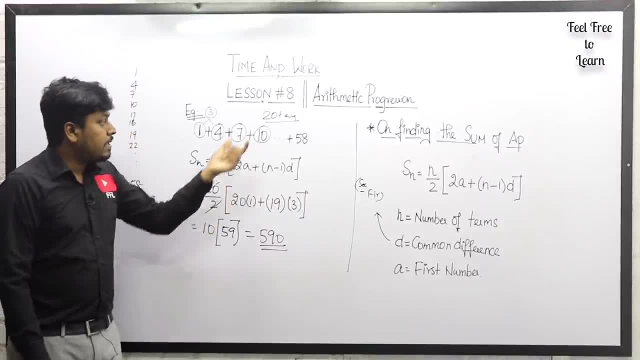 formula and you will find the answer understood. only thing is: the value of n will be given in the question. while reading time and work question, we can able to find what is the total number of terms that are there in the question. so number of terms here. so by using that, we will substitute the value of n. always remember that. 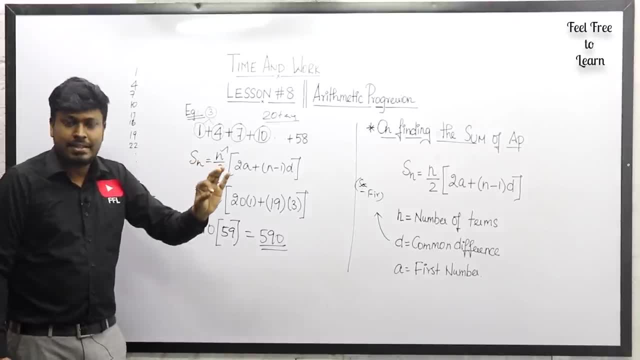 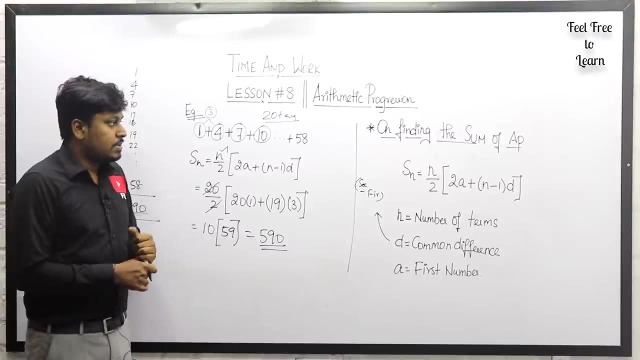 the d is the difference, so which we usually call it as a difference, but while solving, remember second number minus first number will be the value of d understood, and a will be the first number understood and the value of a will be the first number. that's it. so now let me move on to some. 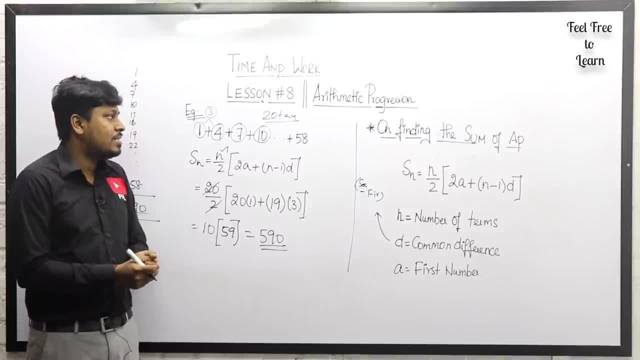 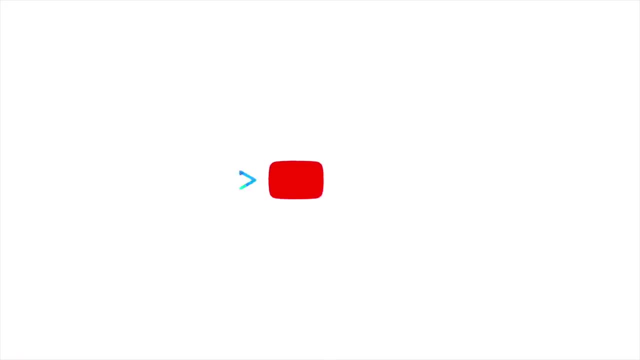 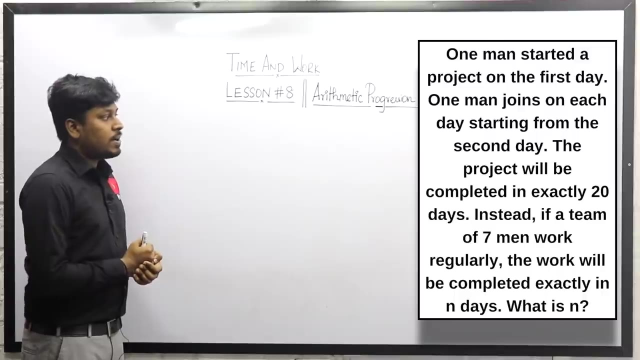 of the example questions on this ap logic so that you can able to understand how to apply the values in the formula. so let me move on to question number one. so question number one: one man started a project on the first day. one man joins on each day starting. 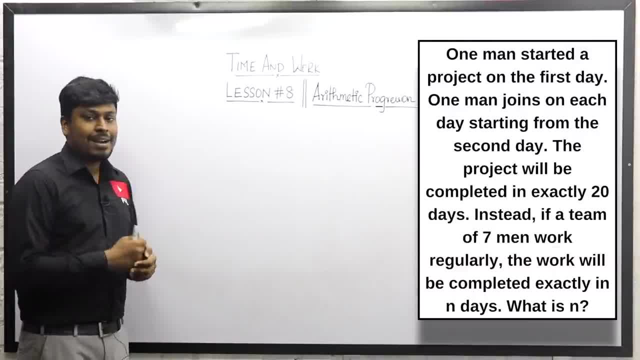 from second day, the project will be completed exactly in 20 days. so instead, a team of seven man worked regularly. the work will be completed exactly in how many days. so just see a friends. let me understand what is the concept of the question. so one man started a project on the first day, so from the second day, 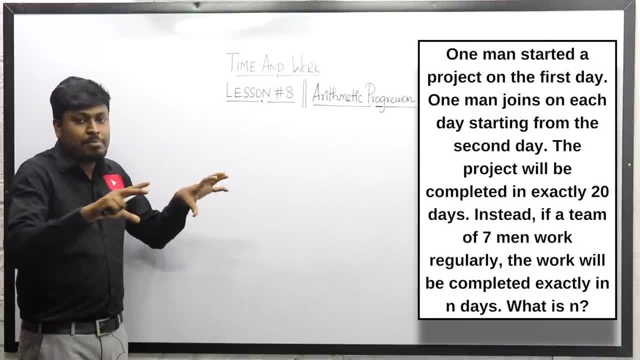 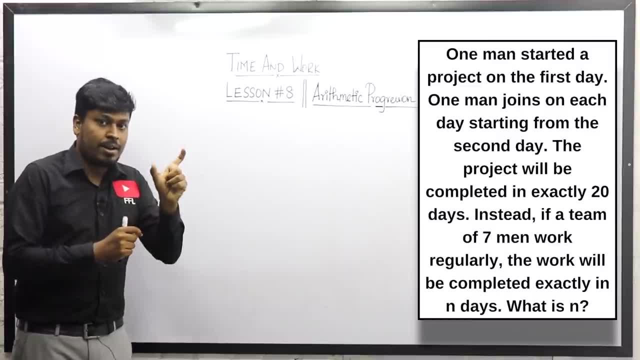 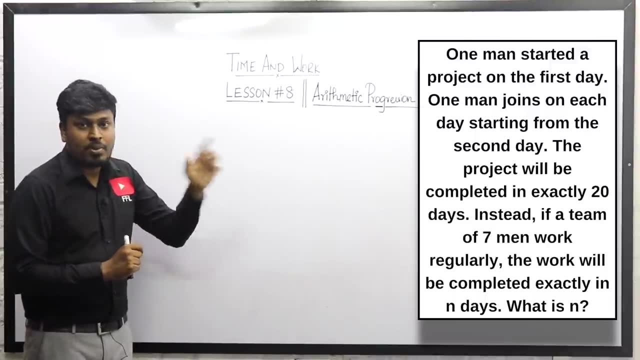 one man is adding right and finally the complete projects. it gets completed on 20 days. and what is our target instead? right the same work if only seven man was doing. how many days the project gets completed? so, initially, one man started the project on the first day, right. so on the first day, one man started the project from the second day. what? 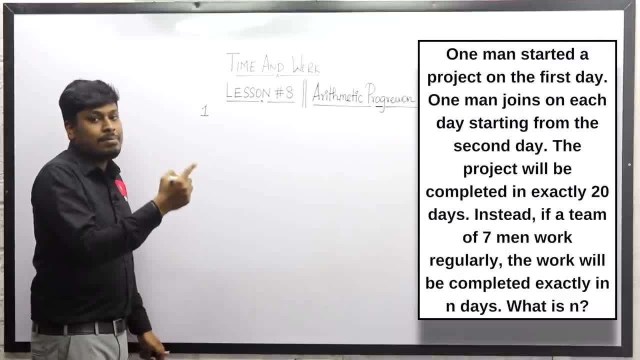 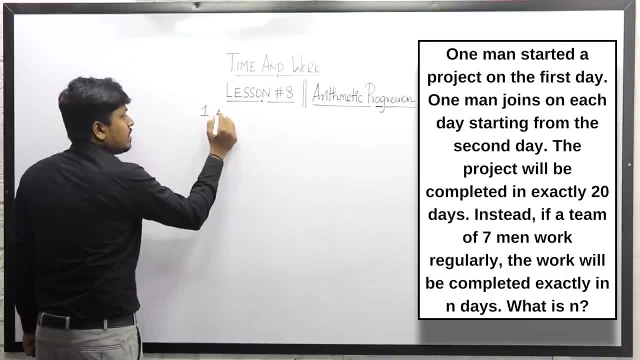 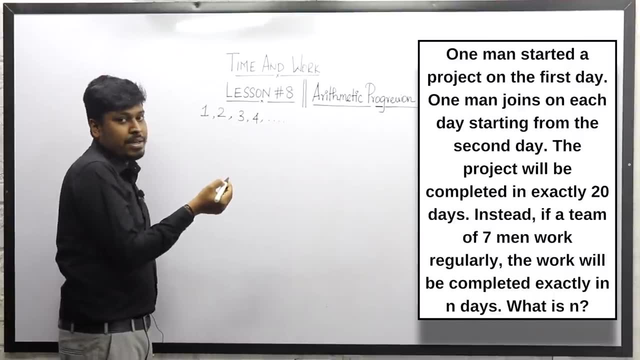 they're saying one man joins on each day, starting from the second day. so definitely we can say on the second day already one man is working on the second day one man joined, so on the second day two persons, third day, three person, four day, four person. so it goes on till the project get completed and 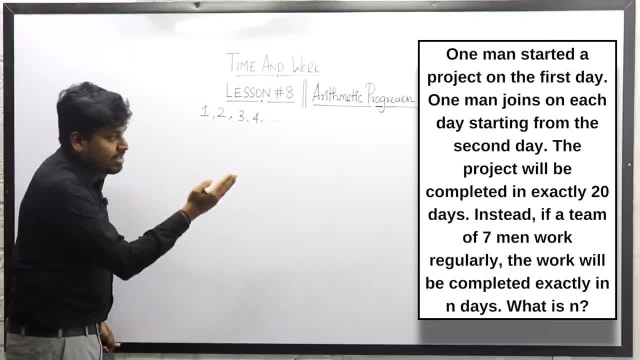 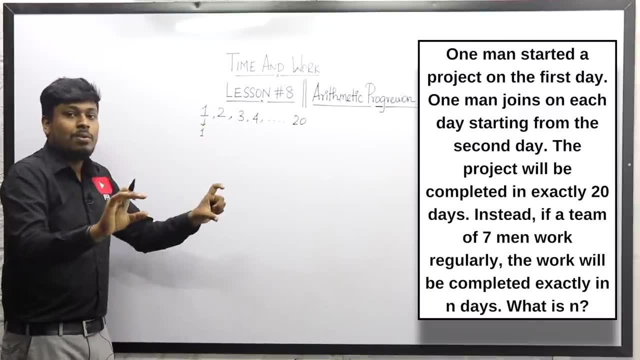 we know the project get completed on the 20th day. just read the question: the project will be completed in 20 days. so totally, they worked for 20 days. so here let me assume that one man doing one part of work in one day, some part of work, right, because the total work was completed in 20 days. so what? 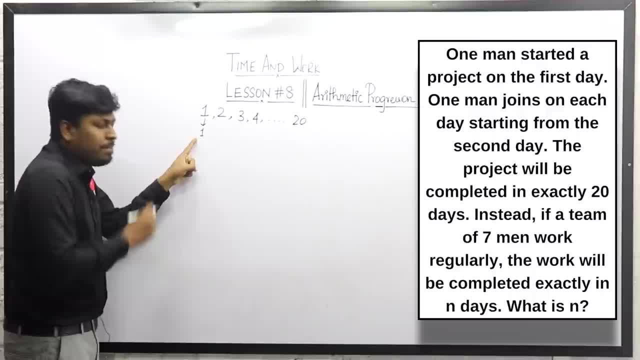 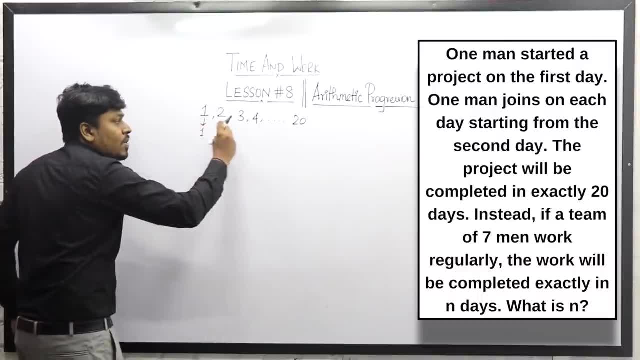 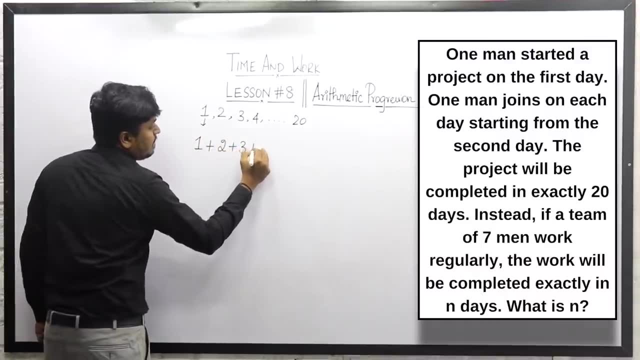 we can do is one day- that is the first day- one part of work is completed. second day, another two parts of work is completed. third day, three parts of work is completed. so it goes on like some pattern. just see here what we can do is one right plus two plus three plus four. it goes on till 20. 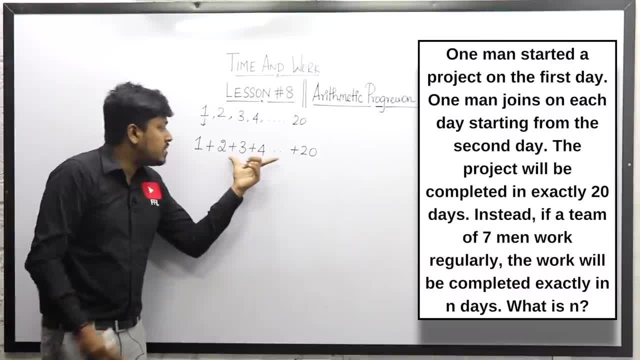 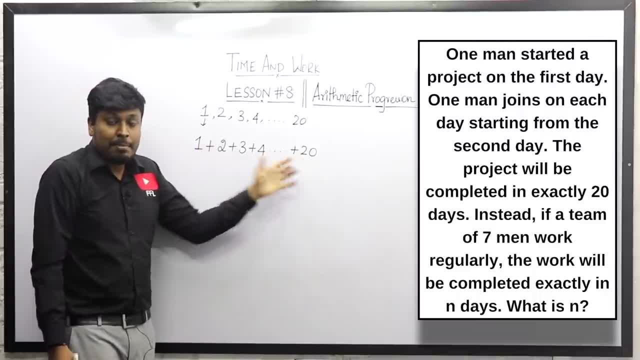 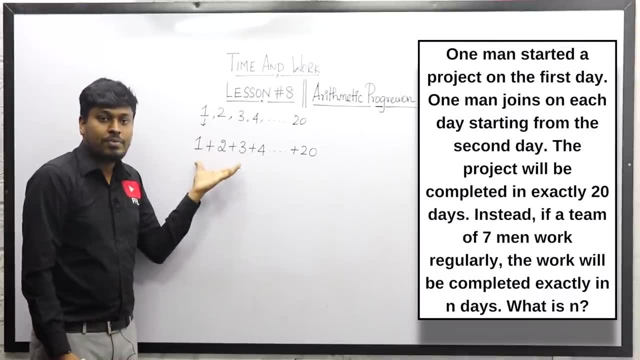 days, because our target to find out of this 20 days total 20 days. how much of work done, right? we don't know. right, the project is completed in 20 days, but we don't know how much work was done. so let me find this the total sum. so it looks like an arithmetic progression. just know, i have. 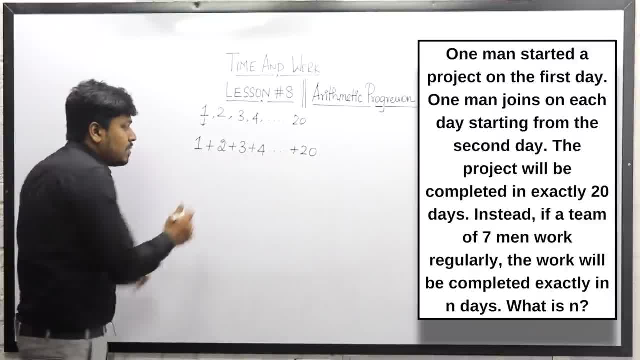 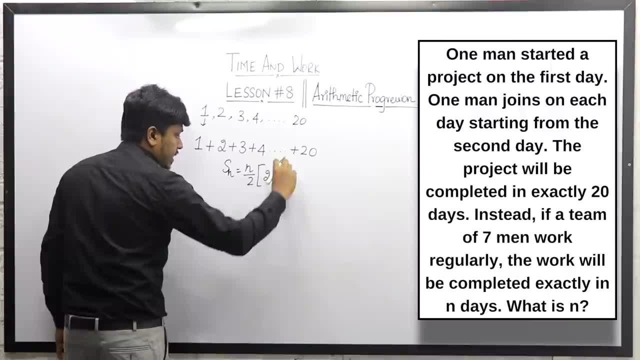 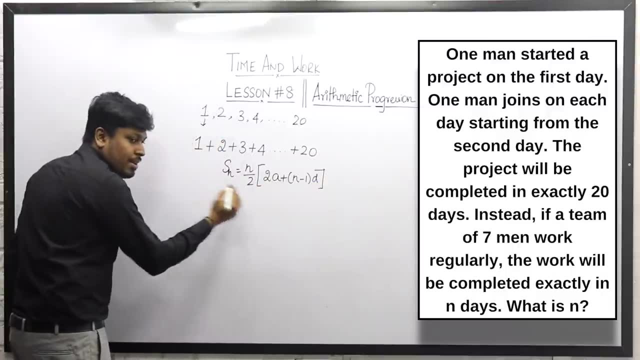 thought you so for finding the total up to 20 we can use a formula that is: s of n is equal to n divided by two into two, of sorry two a. so two a plus n, minus one into d. so substitute all the values in the formula so that we can find. 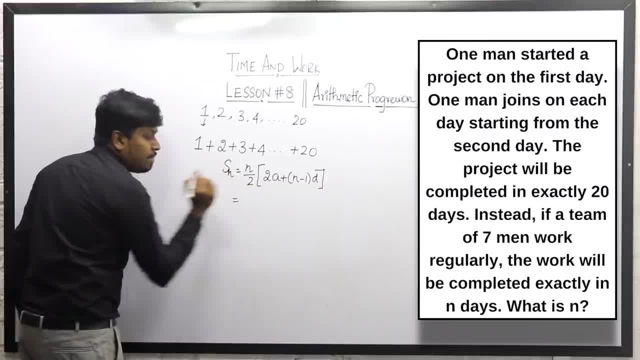 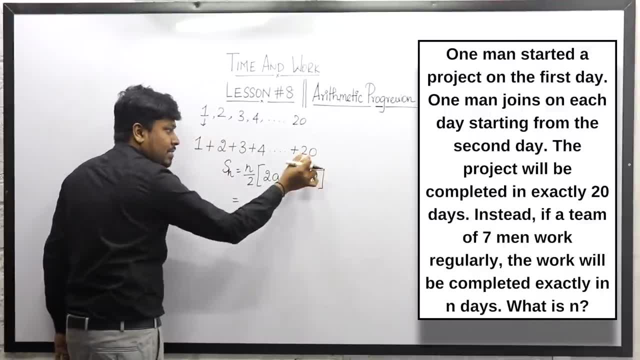 what is the total work done in 20 days? right, so n by two, so the value of n will be 20, because starting from one they, the complete project was completed in 20 days. so the value of n will be 20, so 20 by 2 into. 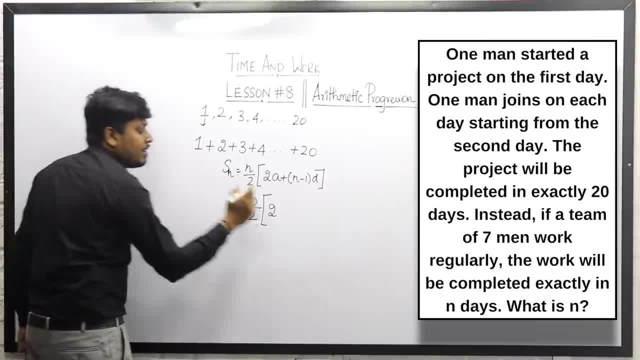 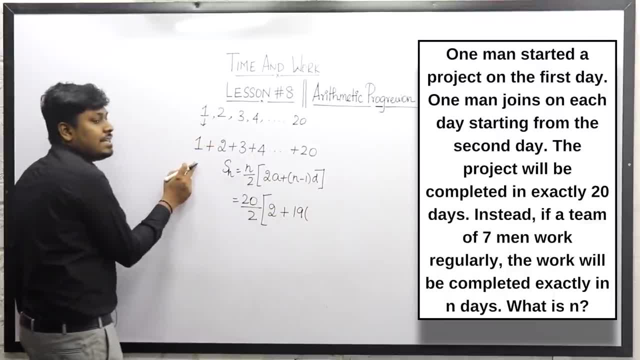 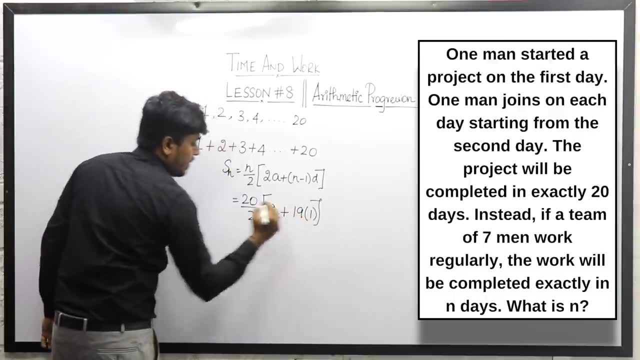 2, 2 of a, so a will be the first number, so a here is one. so plus n minus one, so 20 minus one will be 19 under d. so d is the difference, which means second number minus first number, so second number minus first number. the difference is one, so 21 here. so we can cancel it. this becomes 10, so 19. 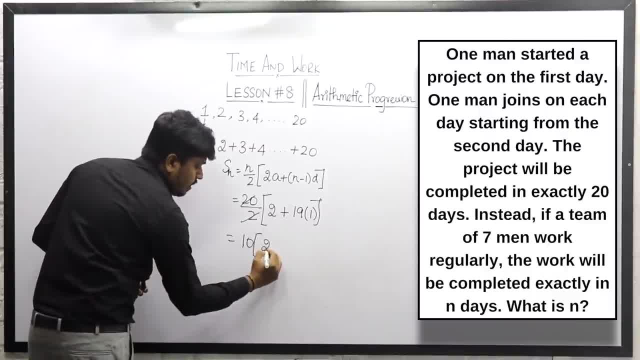 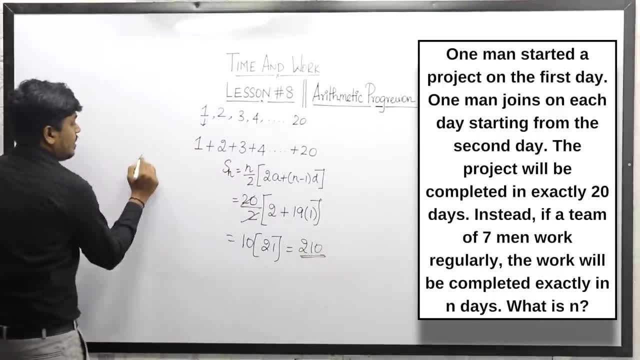 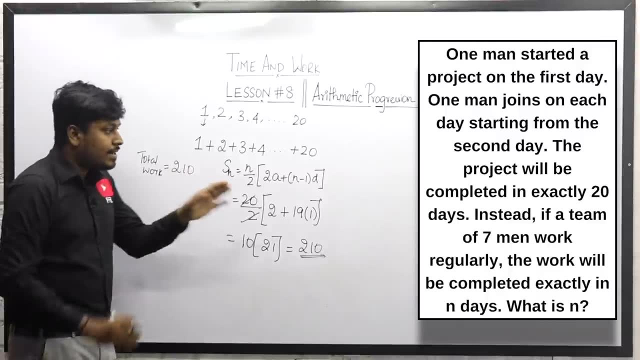 plus 2 will be 21, right, so 21. so 21 into 10 will be 210. so here 210 will be the total work done. right understood, so the total work in this 20 days is 210. but now what is our target at the last, if a team of seven men work regularly, so for doing this work only seven men. 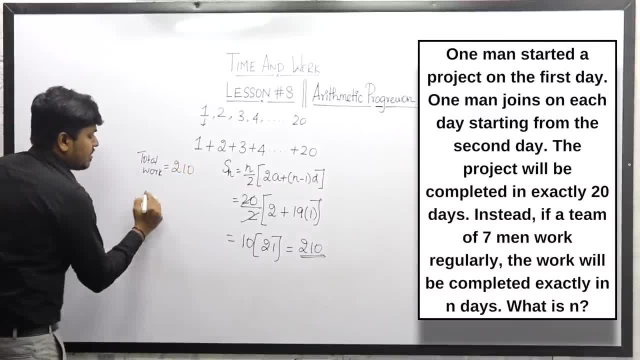 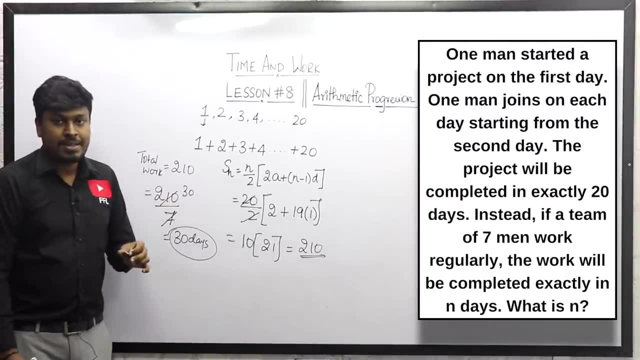 were appointed, so how many days the work will be completed? so usually you can say 220 is the total work, so only seven men is appointed. so if we cancel it 30 days, so only it will take 30 days to complete. so finally, answer for this question number one is 30 days. so here the logic. all are same, what? 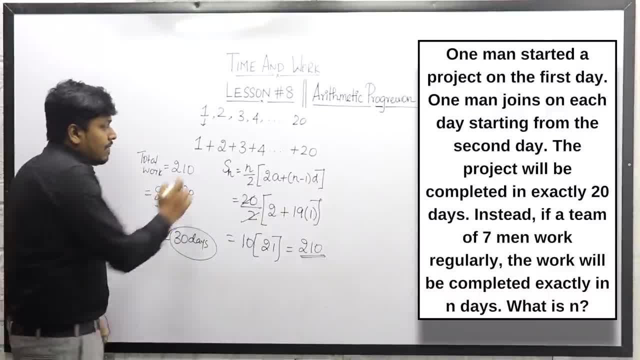 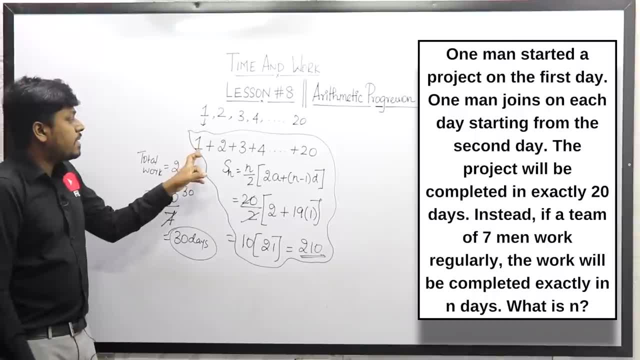 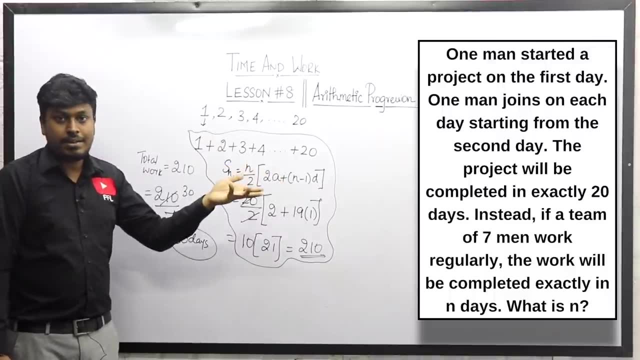 we learned in all the previous lesson. only one thing is we have learned here how to find the total work done, because it is not an easy right one. one part of work done, two part of work done till 20 days. we have to add all the values if it is 60 days. just see how difficult it is if we add. 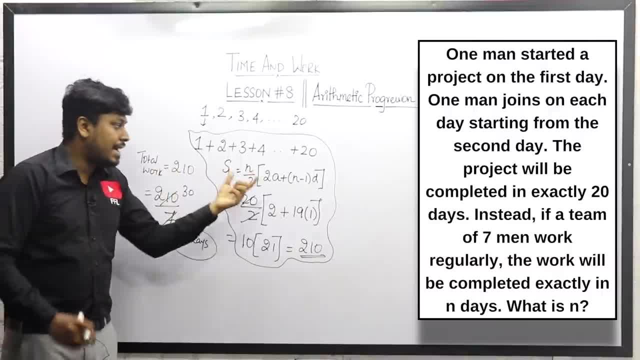 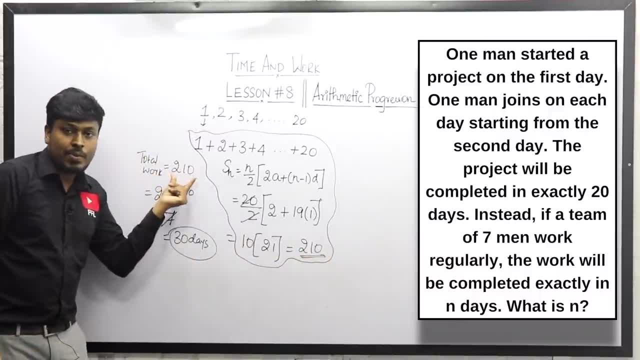 like in a single term. so that's what we have: an ap formula. we are directly substituting it in a formula and we found: what is the total work done in 20 days? so total work done in 20 days is 210. so now our target: this work should be done only by the seven person. so how many days it takes. so 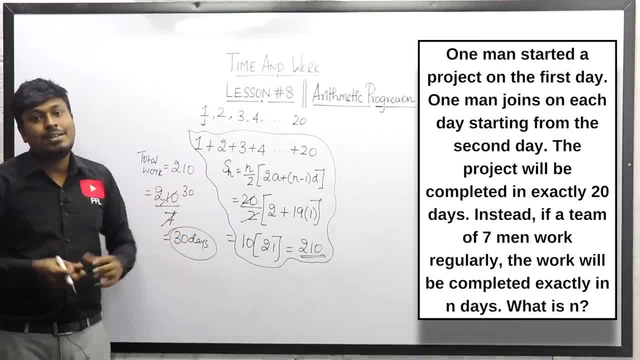 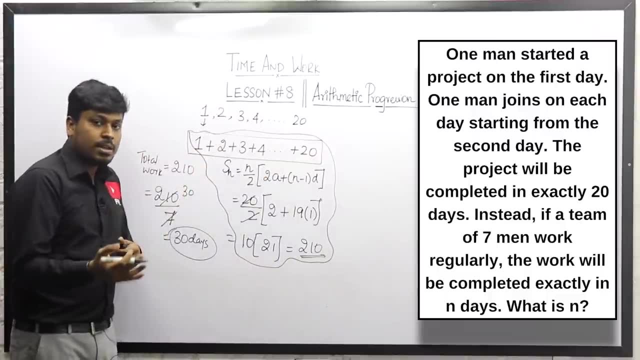 divided by seven. so we can say, we can say that it takes only 30 days to finish the work. that's it understood the logic, friends. so so these are the questions. are very rare question, but listen here, after reading the question straight, to frame this series. right, if you frame this series, then finding the total work done. 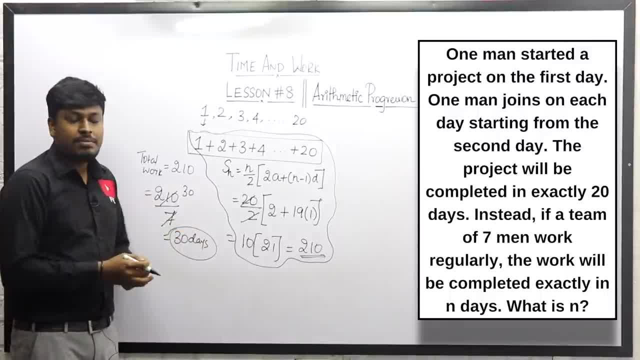 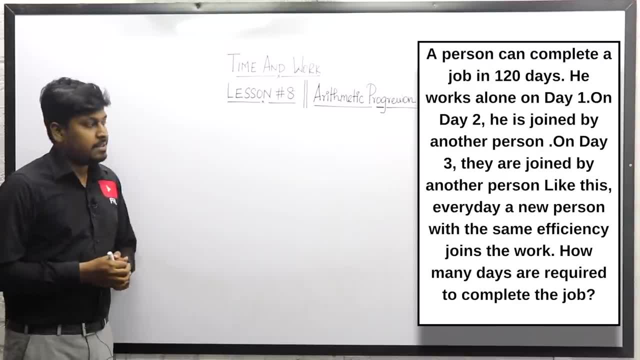 is easy. after finding the total work done, solving a question will be very simple. so finally, answer for question number one, where answer is 30 days. question number three: a person can complete a job in 120 days. he work alone on day one. on day two, is joined by an another person on day three. 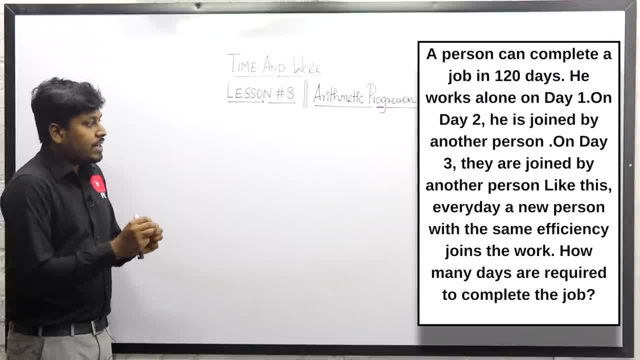 they have joined by an another person, and so on like this. so every day, a new person joins the work with the same efficiency. so how many days is required to complete the job? the friends understood the logic, so what they're saying is: a person can complete a job in 120 days. 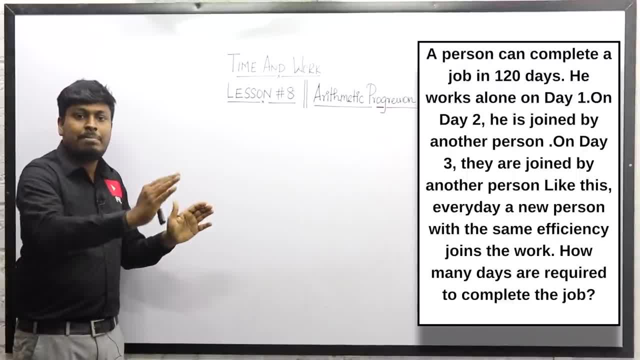 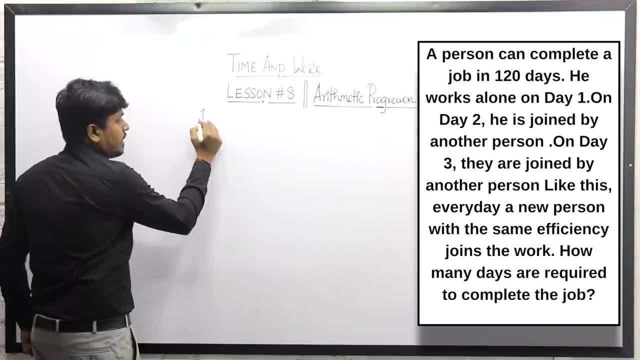 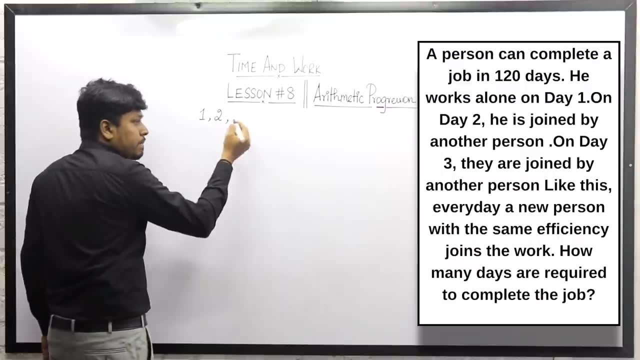 right single person efficiency- one person can complete a piece of job in 120 days- is given. and second thing is he worked alone for day one. so day one one person is working. on the second day he is joined with an another person. so on the second day, two person are working. and on the third day, how many persons are there? three. 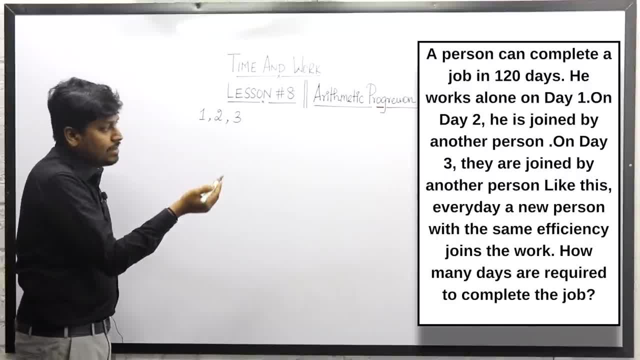 person is working because it's so on right. just see the word again on the day three. they have joined with another person, so it goes on in a logic and the persons that were appointed all are in the same efficiency. so no problem. so what is our target? how many days it required to complete? 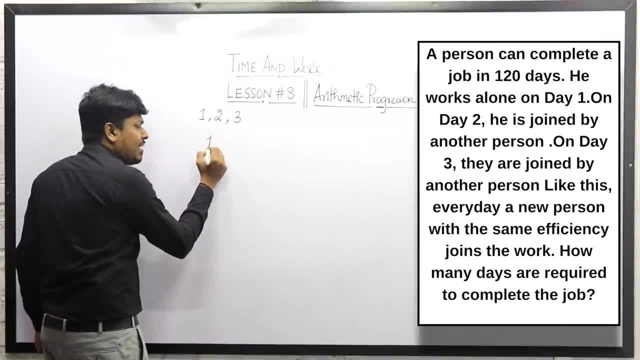 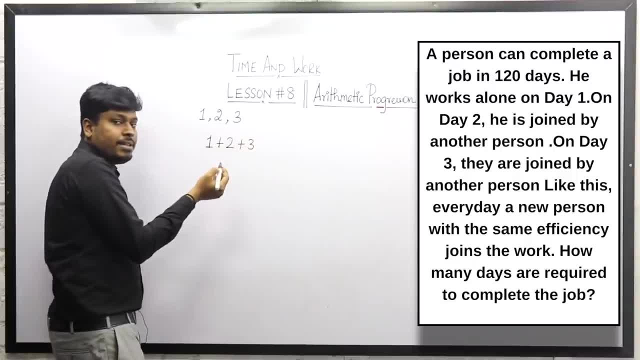 the job. just see here: first day: one person is working. let me assume that one part of work is completed. on the second day, two part of work is completed. on the third day, three part of work is completed by the three person, but we don't know how many days it takes to complete the complete. 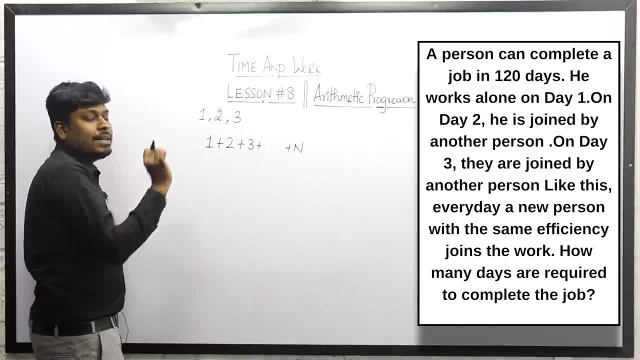 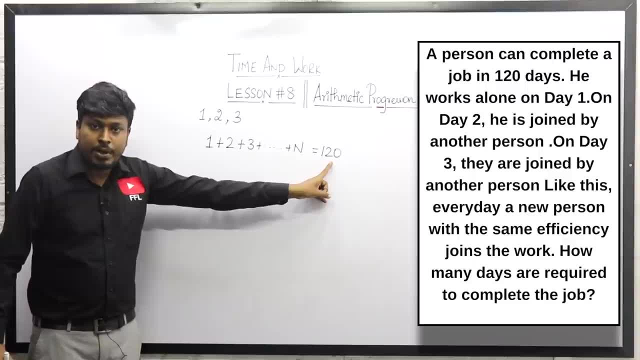 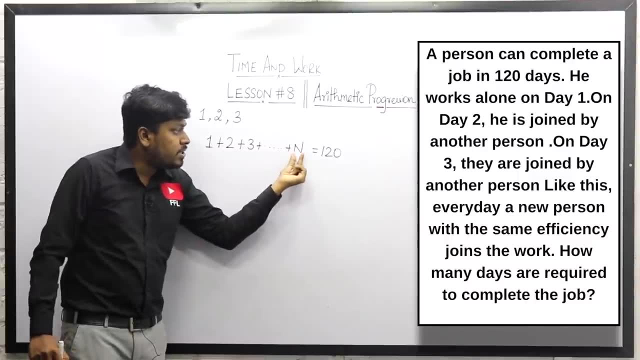 job. but we know that- first point, a person can complete a job in 120 days. so the total job is 120. understood, friends? one person can complete a piece of job in 120 days. that is 120 units of work. so remember that in the previous question we know the total work was completed in 20 days. 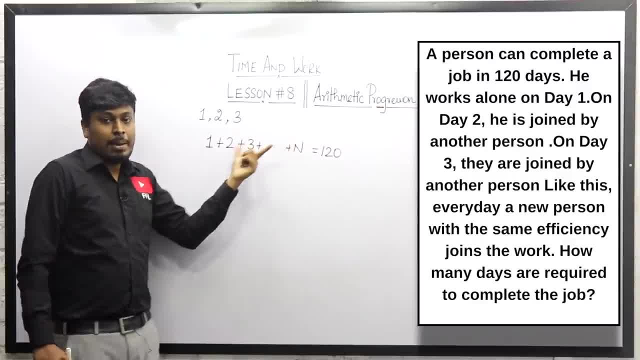 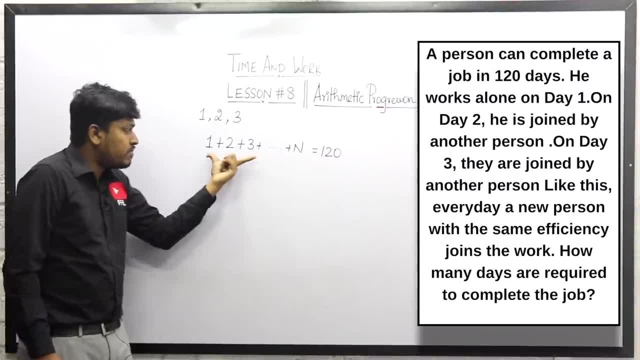 so instead of n we substituted 20 in the previous question. but here we don't know this job, in however many days it gets completed. so here we have assumed n, because the total number of job completed we don't know. that's what we need to find, but one person can complete a job in 120 days. sum of ap. 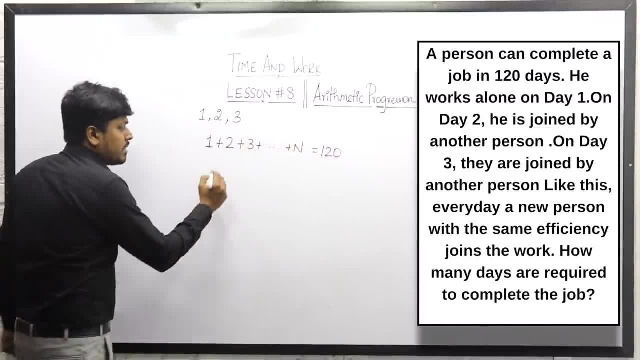 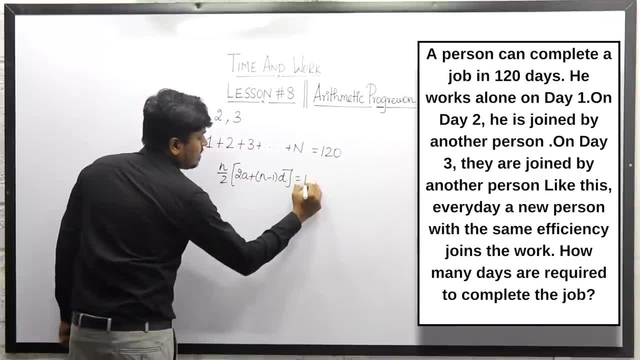 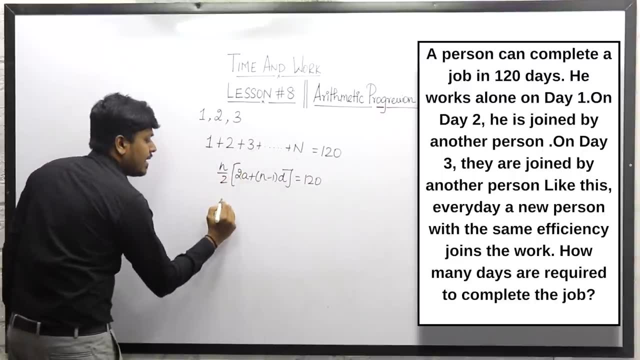 the total sum of ap will be here, right? so same thing. substitute in a formula that is n by 2 into 2a, plus n minus 1 into d is equals to 120, right? so we don't know what is the value of n because we don't know how many days it takes to complete the work. so let me keep the n as it is. 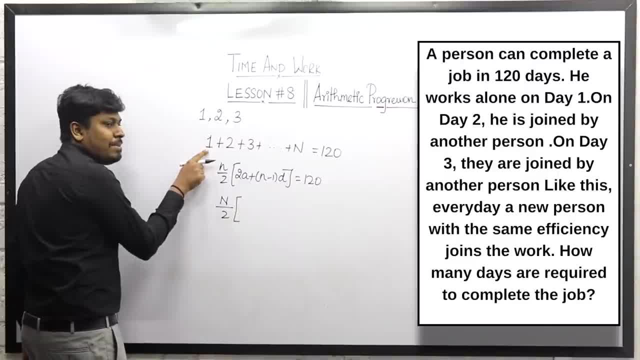 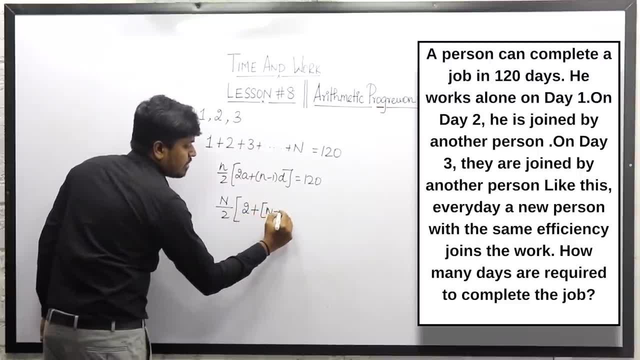 so n by 2, 2 into a, so a will be the first number. so first number is 1. so 2 into 1 will be 2, so plus. so here also we can say that n minus 1 and d will be the difference. so second number minus. 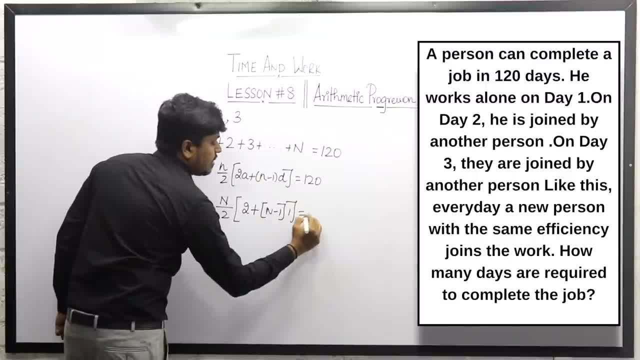 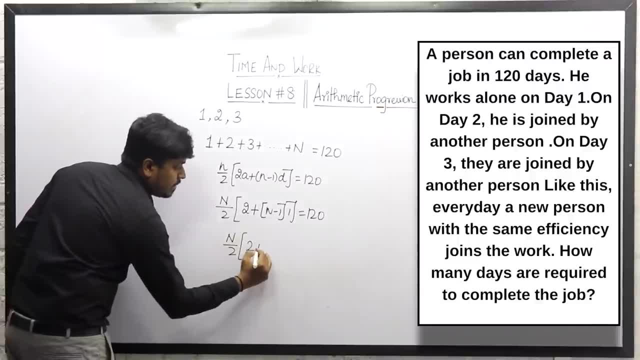 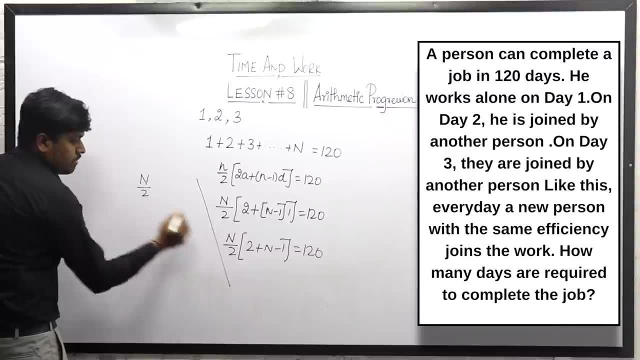 first number. so 2 minus 1, the difference is 1 is equals to 120. so now we need to solve this. so n by 2, so here we can say: 2 plus n minus 1 is equals to 120. so so so n by 2, so n plus 1, so n plus 1 is equal to 120. so finally, n into n plus 1 is equal to 120. 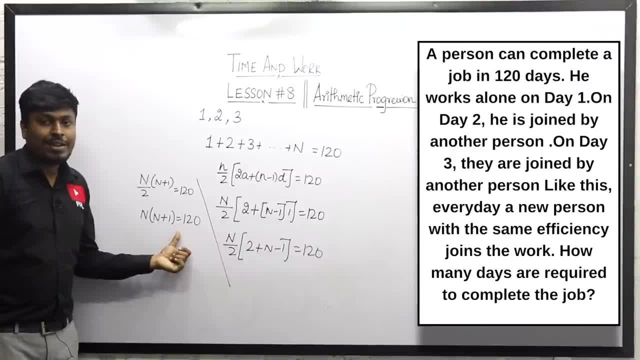 just see here, either you can solve this equation, you can find the answer, or else what we can do is, instead of n, if i substitute 15 here, right? for example, i'm saying: if for n, if i substitute 15, so 15 plus 1 will be 16, so 15 into 16 will be 120, so i'm saying that the value of n is 15. 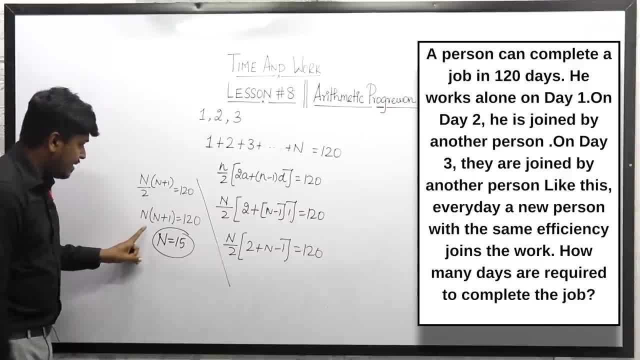 understood, friends. just equating got the logic right. see here here: n into n plus 1. again, just make a note: here n plus 1 is equal to 120 into 2, which is 240. right, we need to multiply this 2, so 120 into 2 will be 240. now either you can solve this equation like this: so n square plus n minus. 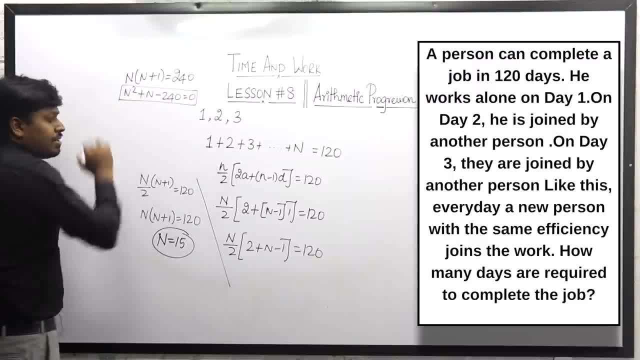 240 is equal to 0. either you can solve an equation or else you can better think the value, because we know the right hand side is 240. so instead of n plus n minus 240 is equal to 0. so instead of n of n, if I substitute the value 15, right. if I substitute n is equal to 15, n plus 1 will be 15. 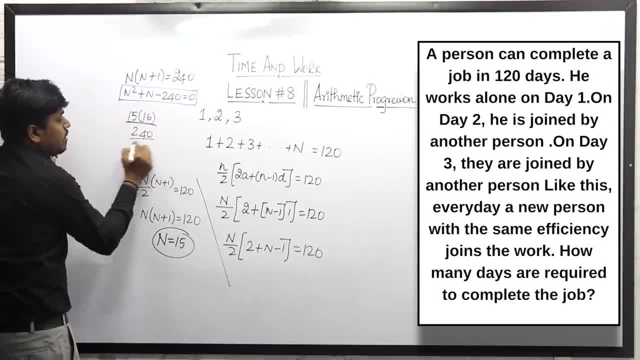 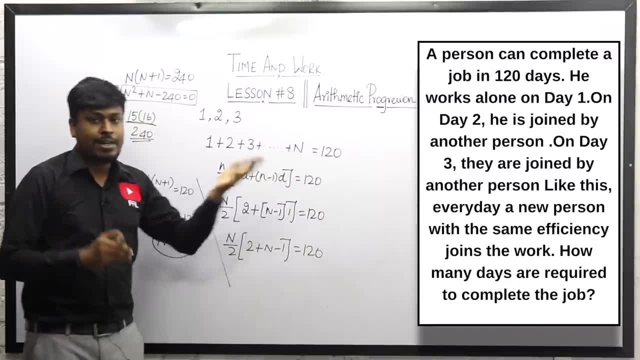 plus 1 will be 16. if I multiply both the values, I am getting 240 right on side value. So that is what I am saying. the value of n is 15.. So, totally, the job is completed in 15 days. So the answer for: 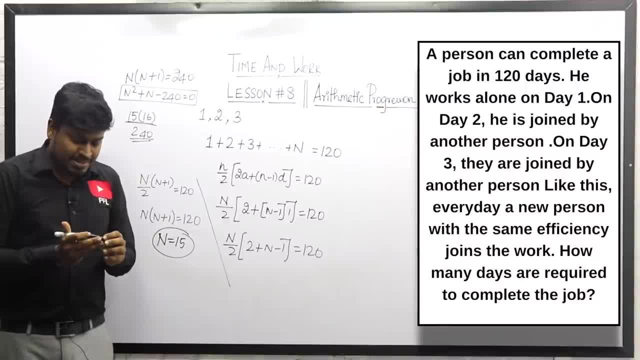 question number 2 is 15 days, understood? It is very easy, right? you should know how to write this pattern and also how to apply this in a formula. So that is it. So, friends, understood. So this will be the answer for question number 2, where the work will be completed in 15 days. So, friends, here is. 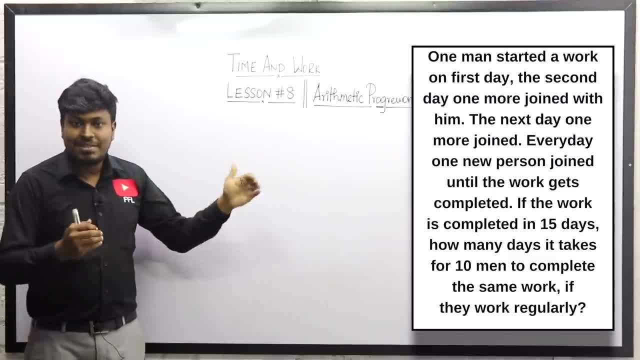 question number 3.. So try to solve this question number 3 as a Omer question, I think. after reading this question, try to find whether the value of n is given or value of n is not given. I think this question is based on the logic. question number 1, right? So we need to find the sum of the total ap. 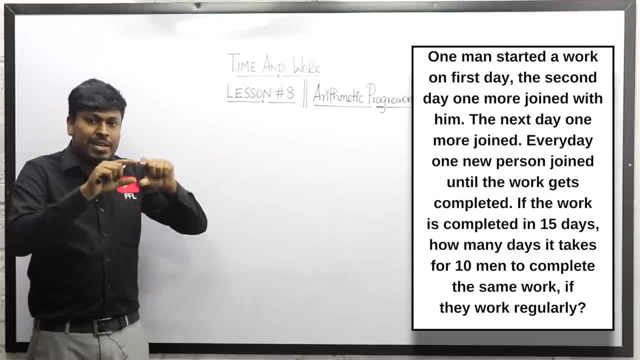 So usually you know After reading this question, you need to frame that order sequence correctly. So once you frame that sequence correctly, solving a question is very simple. So, friends, that is it about this, lesson number 8.. So here the lesson number 8 is very small lesson, but remember that if you are preparing 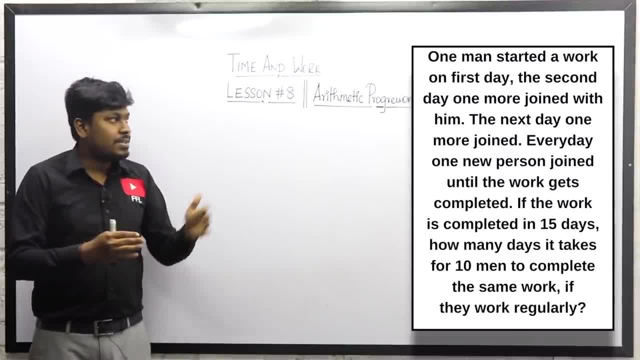 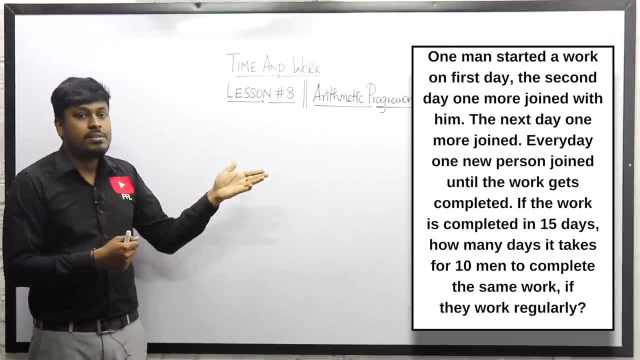 for any competitive exams in quantitative aptitude section. that is time on work. you should know all the logics, So that is what I have taught this in lesson number 8.. You know these are the questions that was asked in GMAT exam previous year 2017..